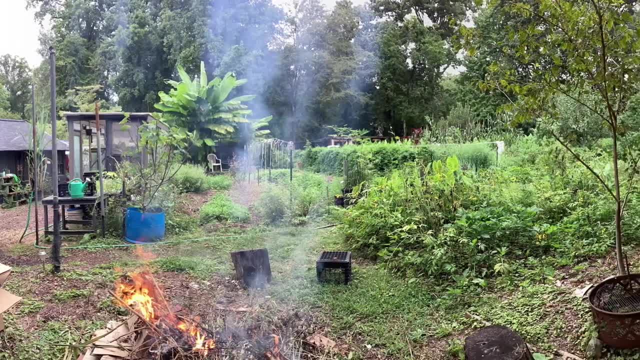 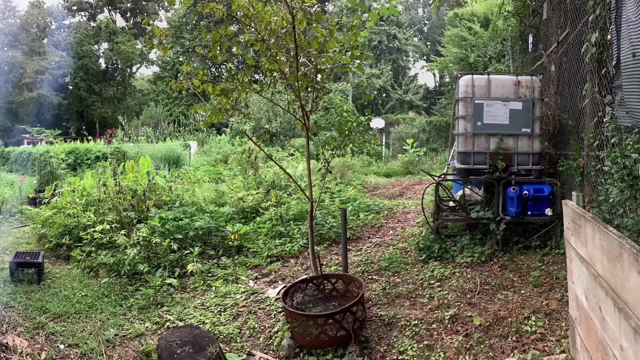 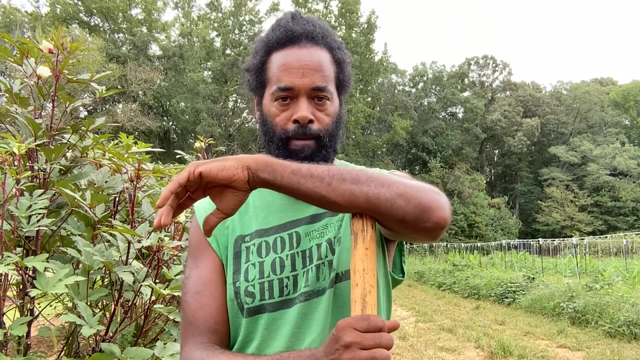 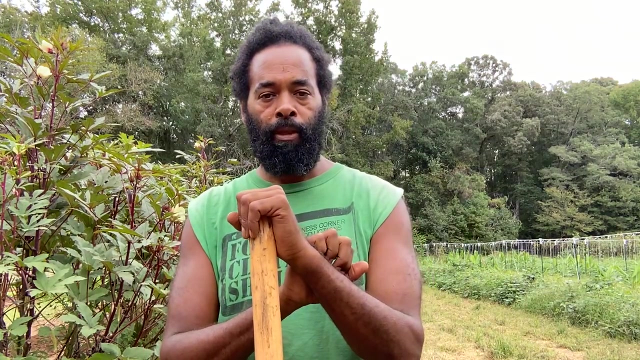 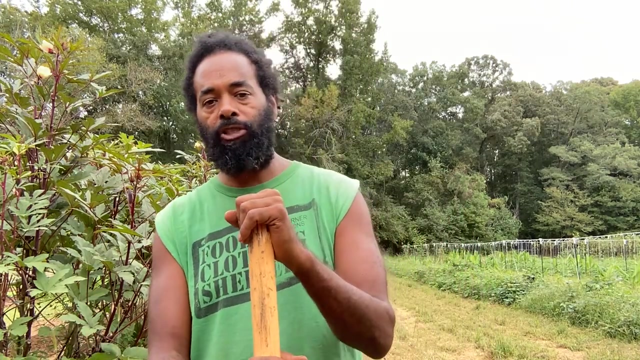 When we look at the differences between urban agriculture and rural agriculture, right In urban agriculture, we often have to contend with the fact that in urban cities there's real estate concerns, real estate, money concerns, financial concerns and highest and best use. 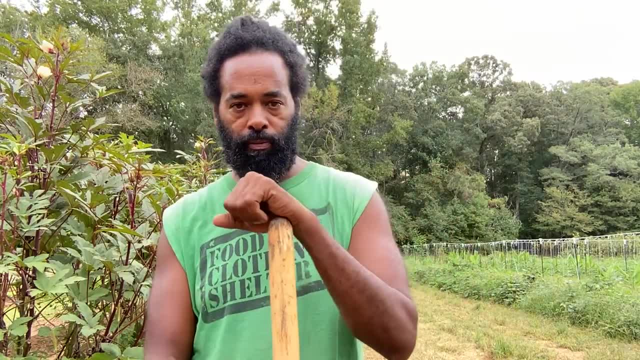 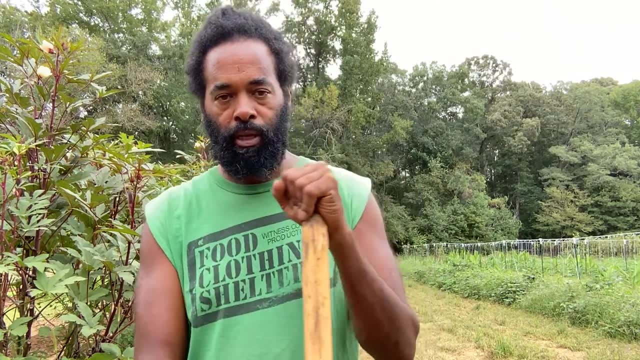 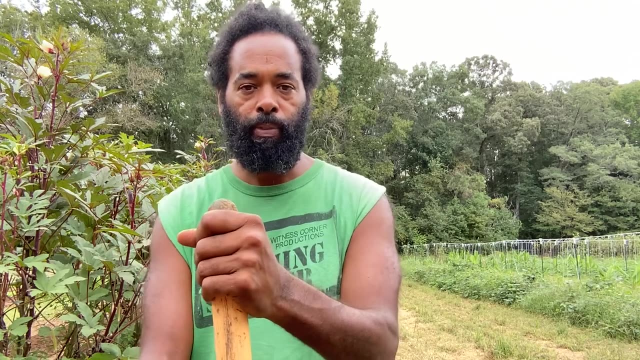 So what is an acre of farmland going for? nowadays? Around $13,000 an acre, Used to be about $7,000 an acre, And we know that there are people who've been buying up farmland- different tech people, different billionaire class people, millionaire class. 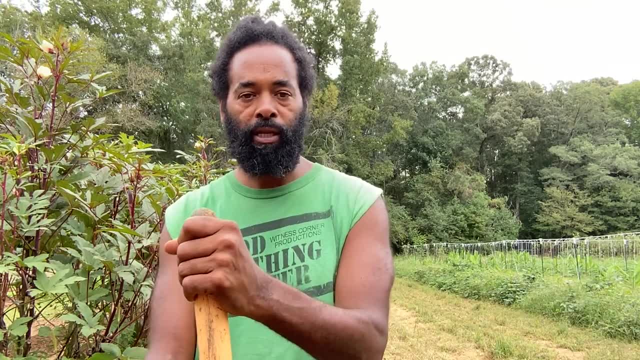 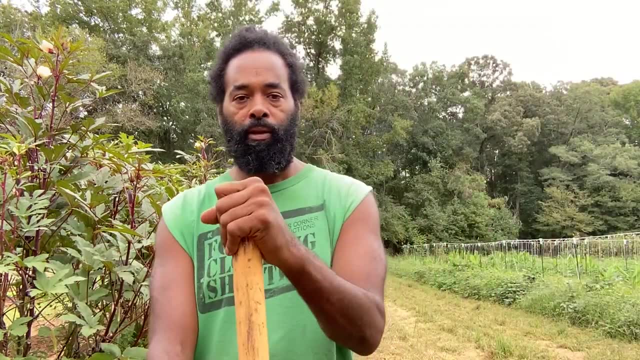 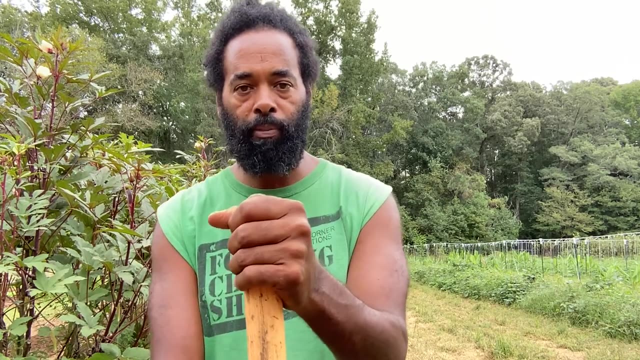 And when they're buying up farmland, it's not because they want to become farmers, at least not in the way you might think. They may be interested in robotics, They may be interested in lab laboratory food, They may be interested in subterranean water, rights of the farmland, and not necessarily. 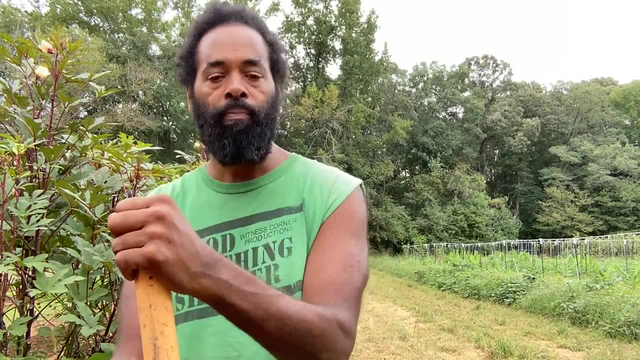 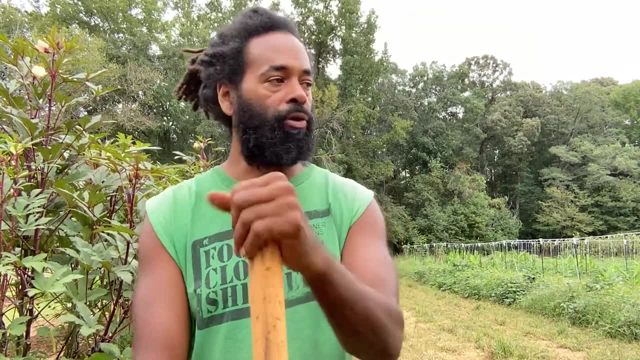 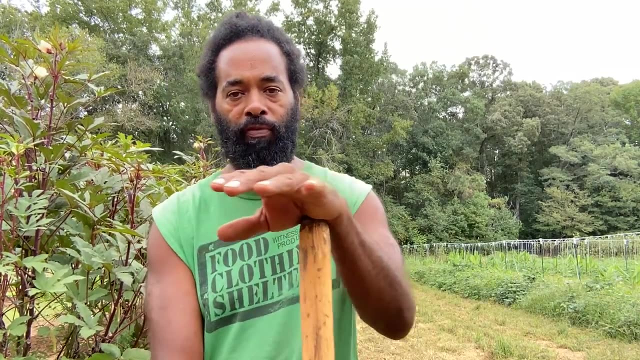 the surface level land, They may not be interested in that at all. So for those of us who are doing farming in urban situations and we are immediately faced with highest and best use, what's the best value I can get for this property, based on being a property owner rather than the farmer? the farmer might 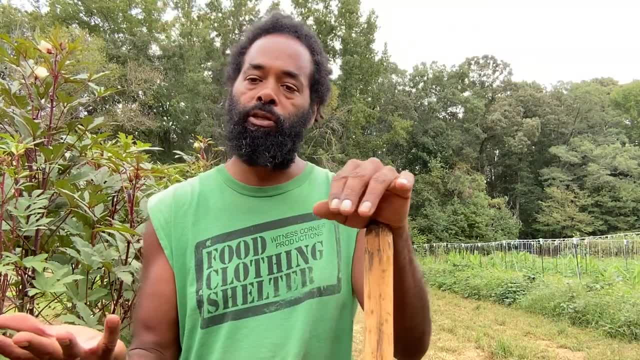 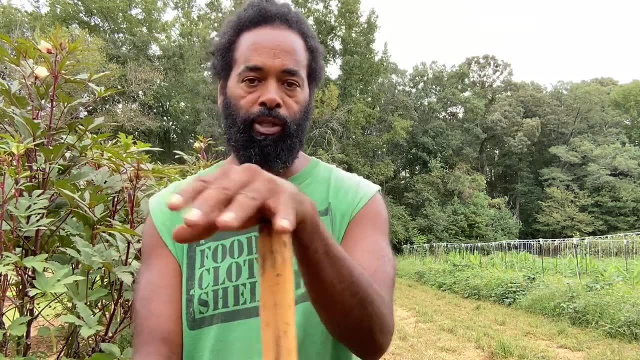 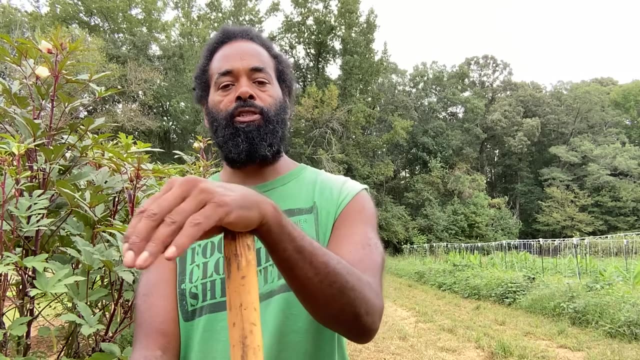 be thinking: how much production can I get from the surface of this property and then take it to market, Whereas the property owner- which oftentimes in urban farming situations, the farmer and the property owner are not the same person- The property owner may be just holding out on. 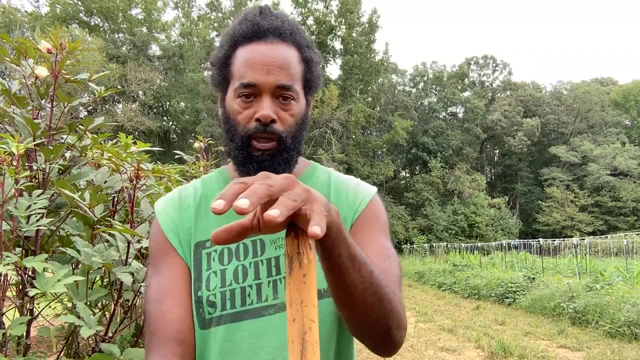 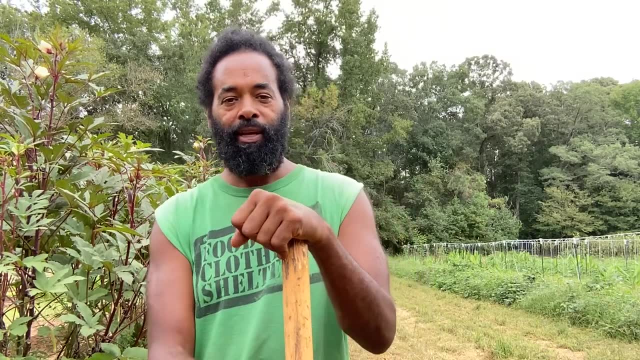 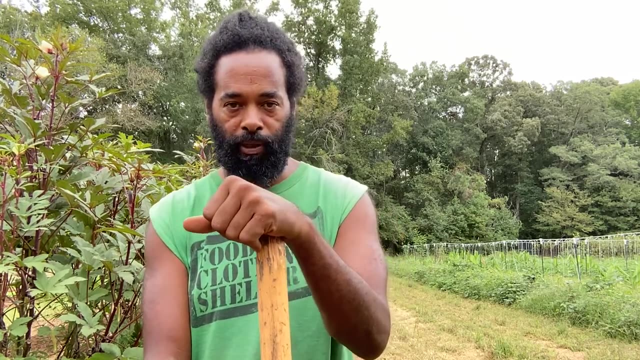 Having somebody maintain the beauty of the property while they're waiting for the value in that area to go up and then they're going to sell. Ironically, it's farms in neighborhoods that bring up or contribute to bringing up the value of the property that then they kind of price themselves out of. 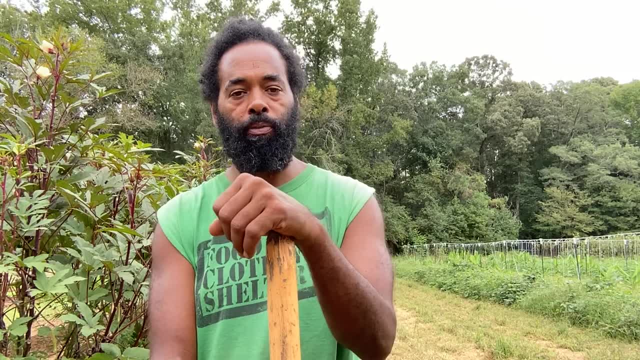 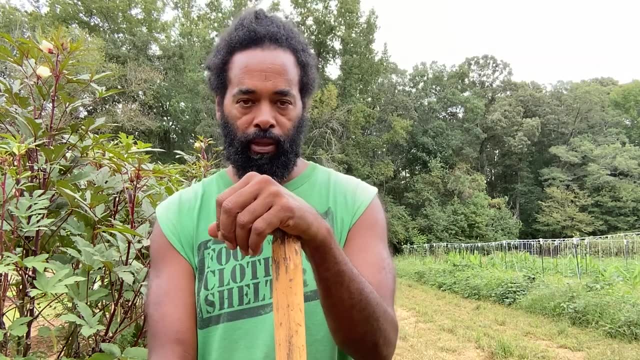 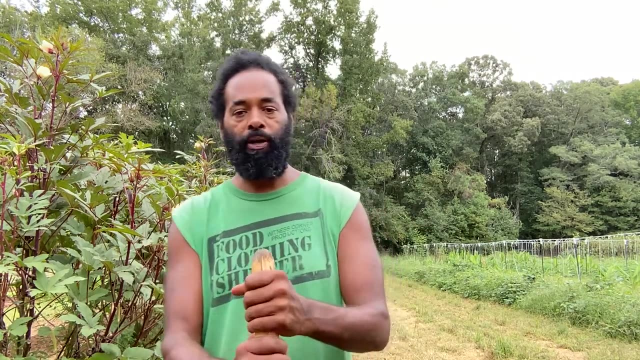 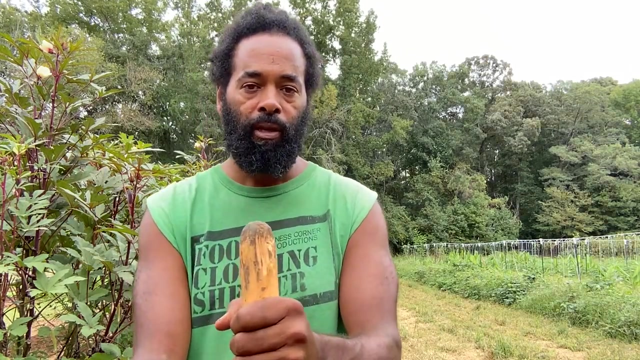 So, having helped to establish multiple mini farms throughout Metro Atlanta, it's become expected that the spaces that we farm will be soon overtaken or taken back by the property owner and utilized for another purpose. Sometimes it's surprising. Sometimes farms have been asked to uproot and move because the property was going to be sold or used. 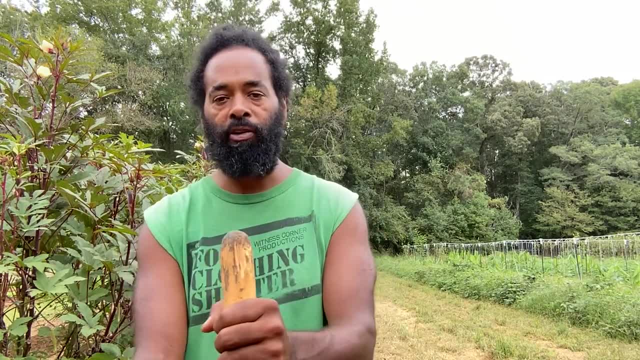 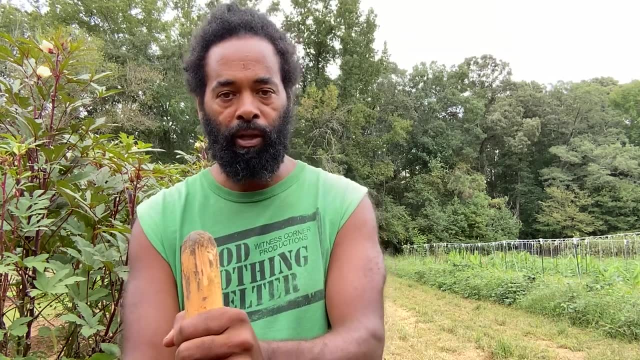 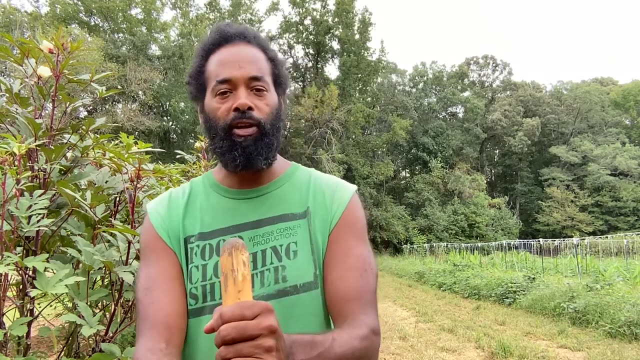 for development and you go by there five, six years later and it's still a fenced up property with no food Growing on it, no development happening on it, but lots of weeds and grass growing and trash and vandalism and different uses that are not highest and best use, certainly not higher than the use of 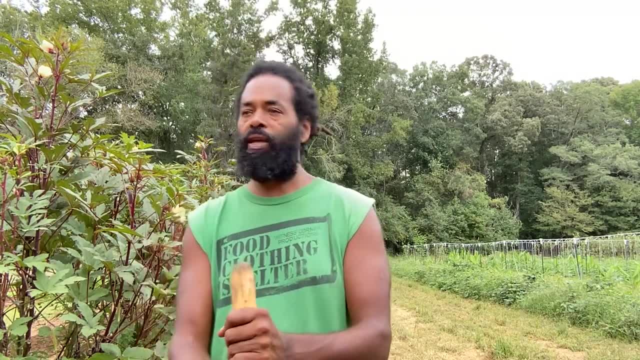 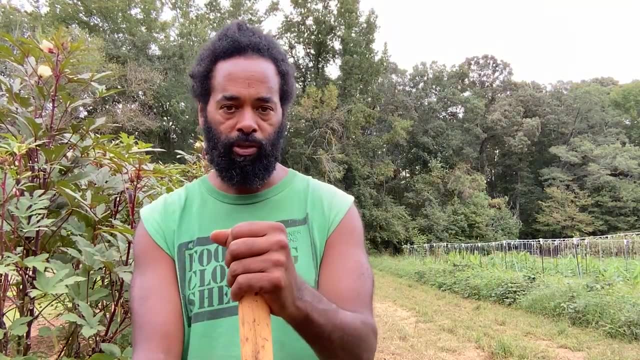 a farm, So why was the farm asked to leave? And then there are situations where people buy a piece of property that has been developed, that was kind of dormant for years, then developed as a farm site, which generated interest around that farm site. 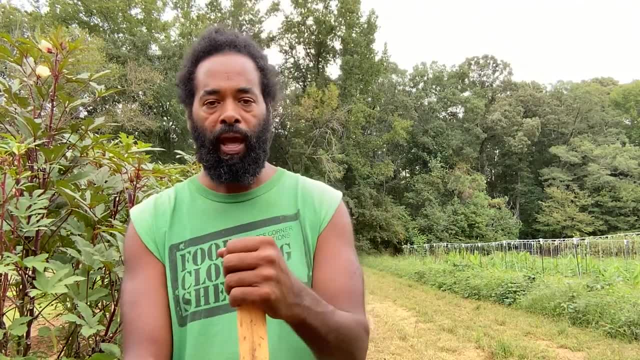 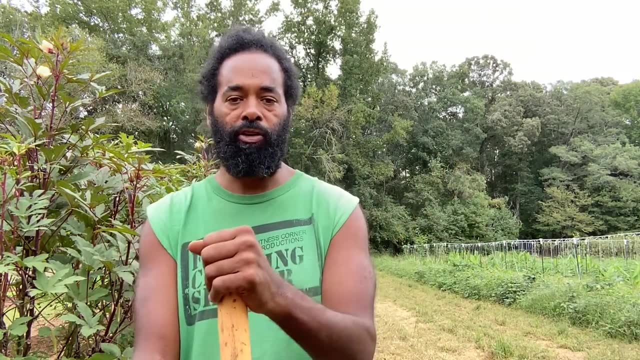 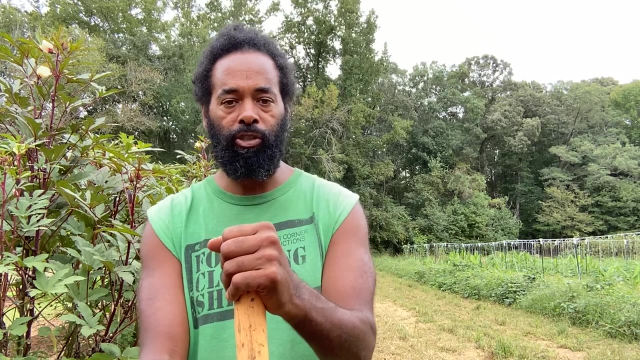 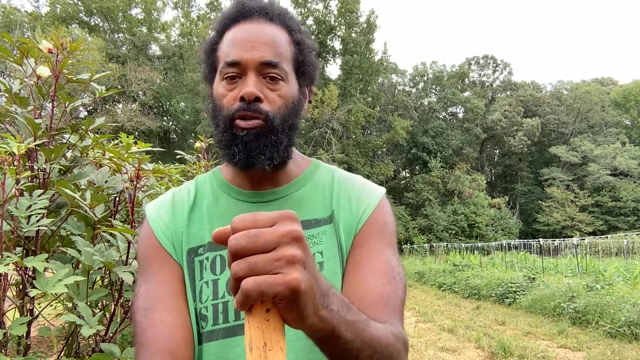 And then New ownership comes in and the space gets paved or it gets covered in sod and turned into something different. in our urban communities There is no shortage of churches, plenty of spas and places to indulge in: leisure bars, hair salons- how much. 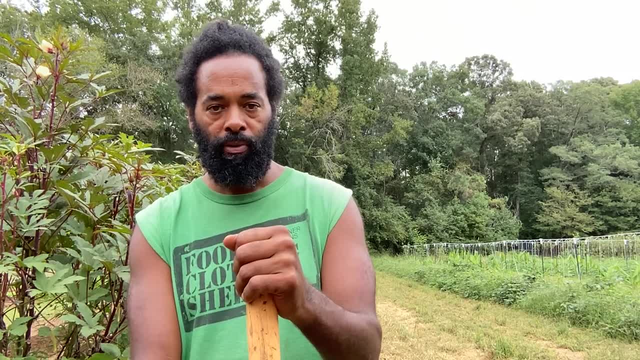 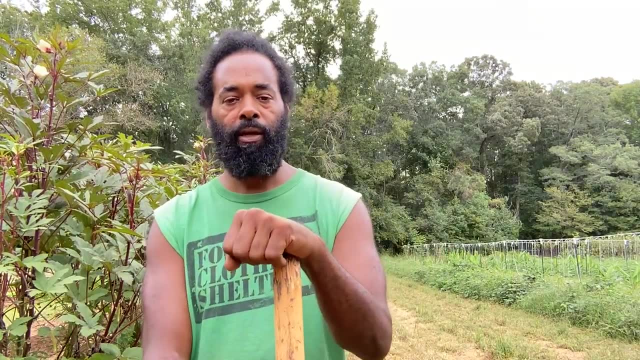 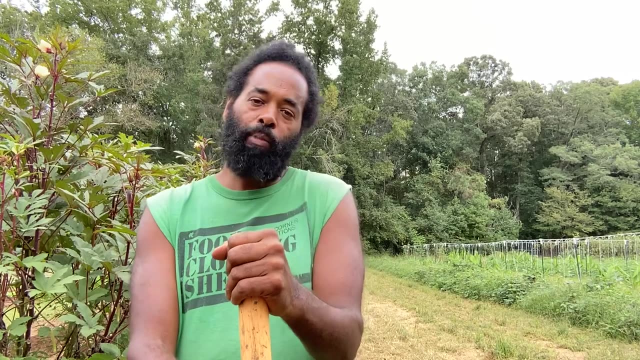 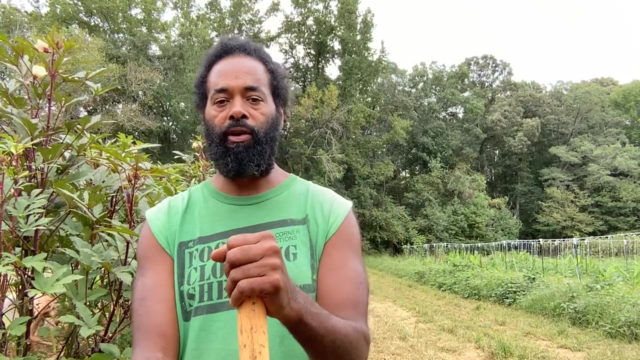 leisure activity do we actually need right now, When we see the global financial system collapsing? should we, as urban dwellers, be engaged in leisure activity, and how much? what percentage of our time? if we have access to land, Many of us who are in in areas like Metro Atlanta- it's still a city and yet there is cultivatable land- 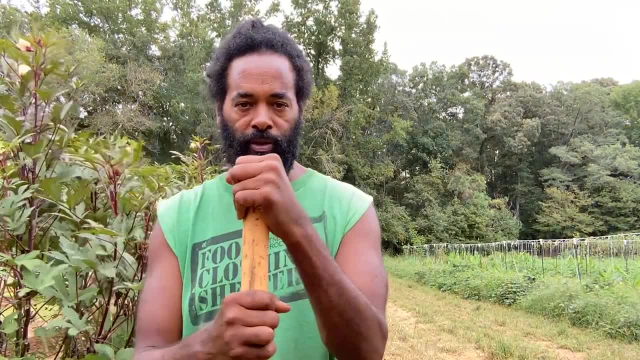 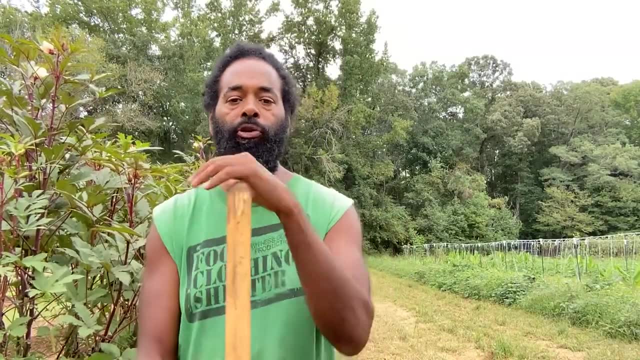 Many of us who are in in areas like Metro Atlanta. it's still a city and yet there is cultivatable earth, oftentimes in the hands of people that are in our own communities, and it's not being cultivated. So there's opportunity there. 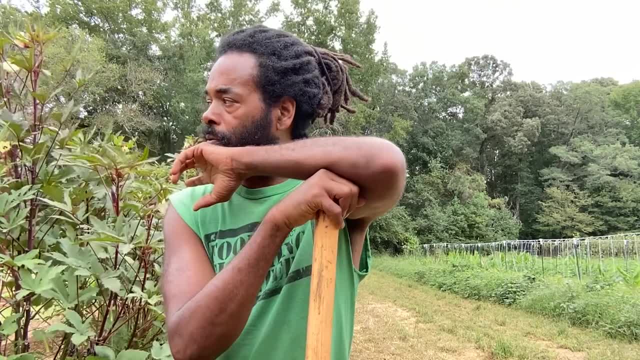 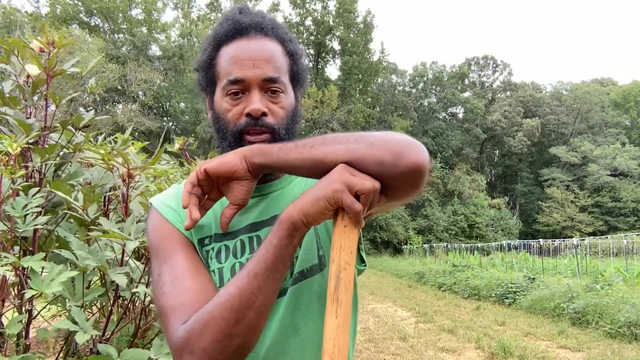 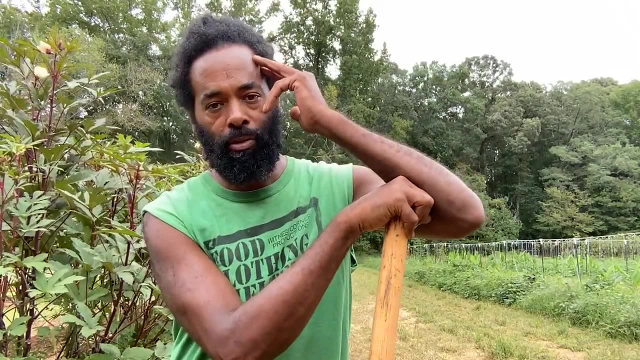 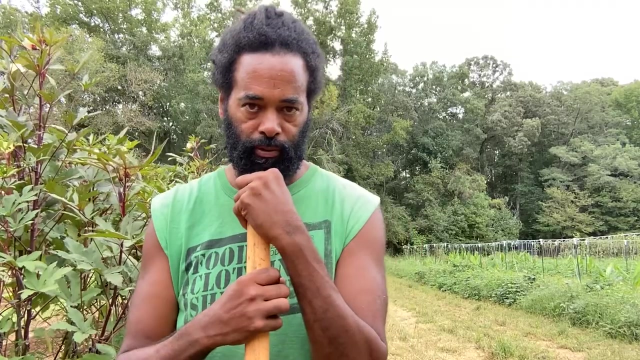 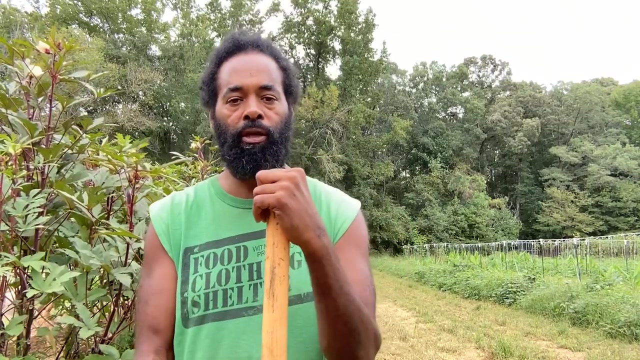 So think about it When we are witnessing and experiencing, many of us deep health issues that could be physical, they could be psychological. These health issues, many of them, are based in malnutrition: malnutrition at the cellular level, where our cells are starved for nutrition because the soil has been treated so bad where our food is produced. 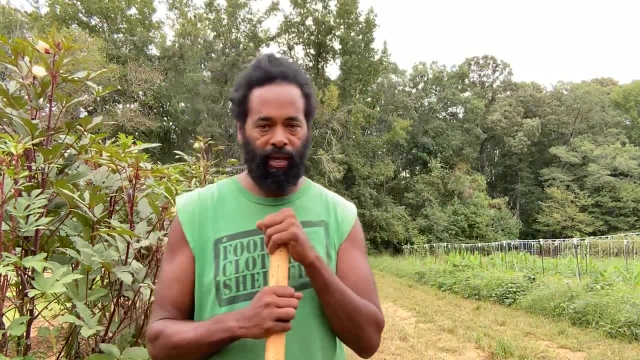 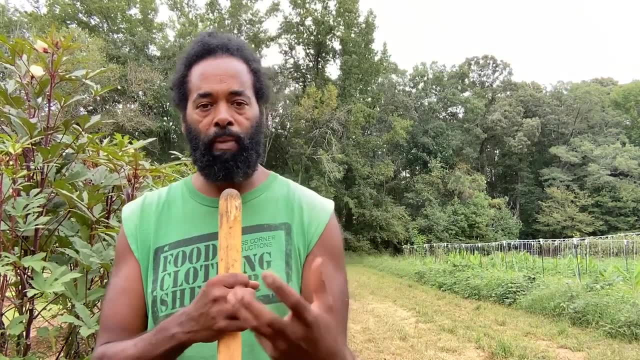 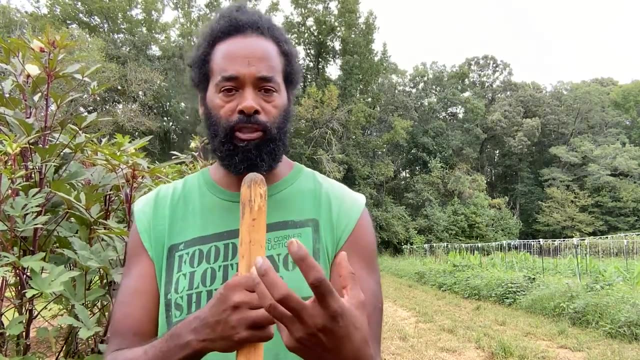 If the soil lacks microorganisms, the body lacks them. If the soil lacks healthy bacteria, the body lacks them. It is these bacteria And microorganisms that help to balance the endocrine system and keep our hormonal system in balance, so that we can then master our emotional bodies. 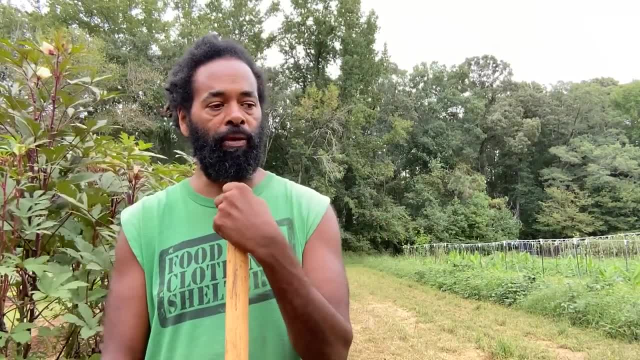 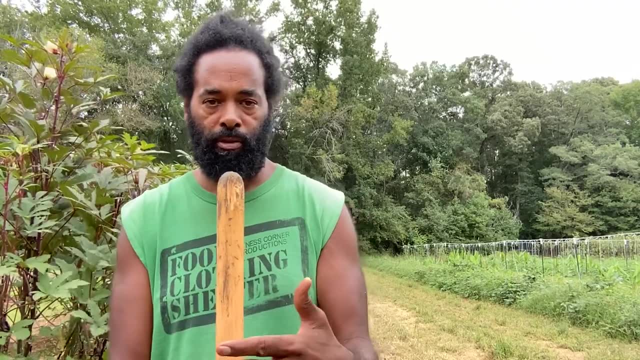 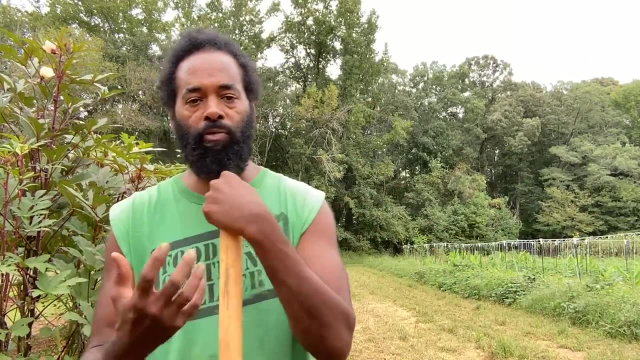 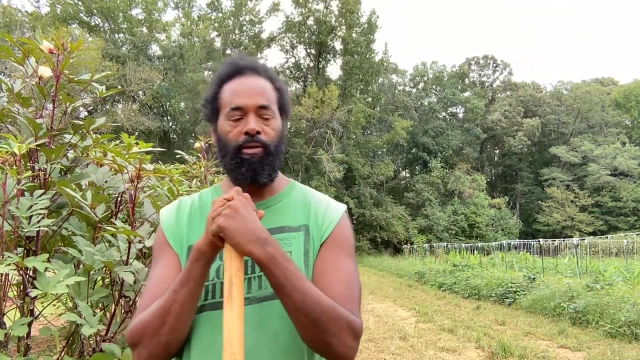 Some people have said that civilization is actually the systematic mastery of human emotions. That's how civilization comes to be: not the eradication of human emotions, But to see and recognize that we have these emotions: loss, trauma, joy, forgiveness, passion, play. we have all of these happening inside of us. 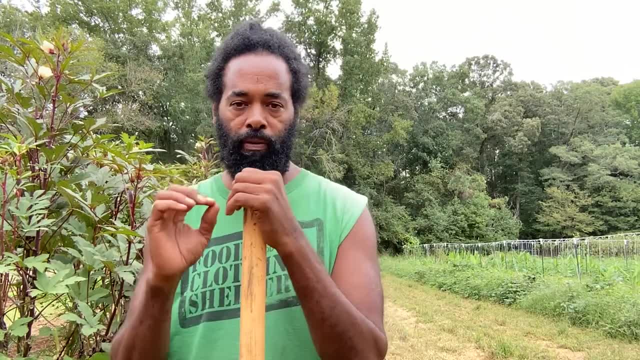 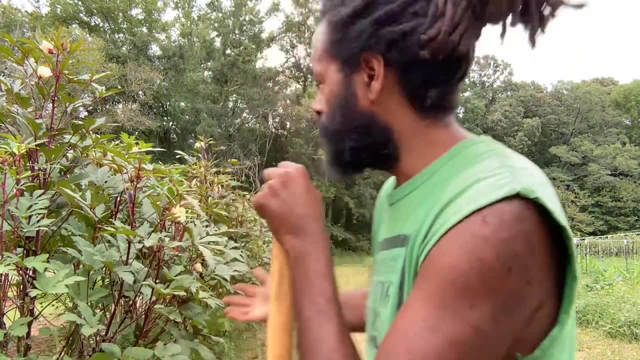 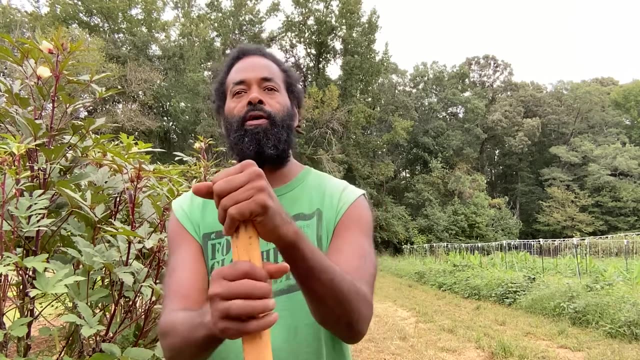 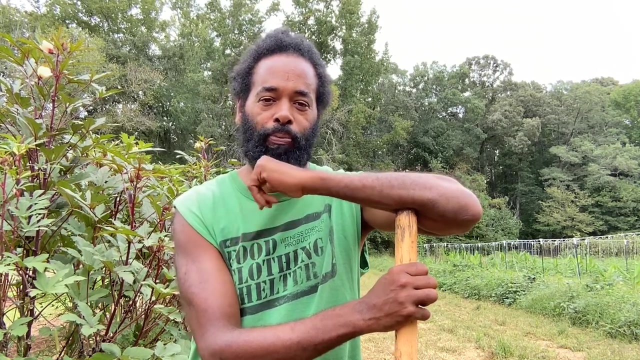 And if we can create systems for utilizing these emotions and mastering these experiences, then we start to have a civilization. Well, agriculture was one of the keys to that, Because when we're out in the, In these spaces, we experience multiple emotions, from being elated and proud to being disappointed and hurt. 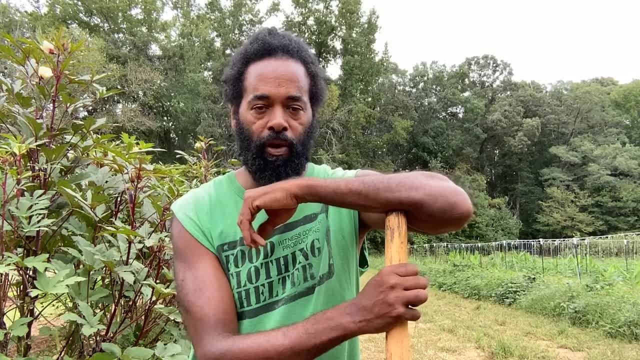 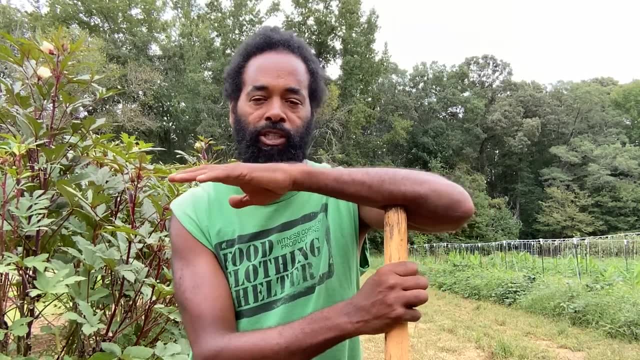 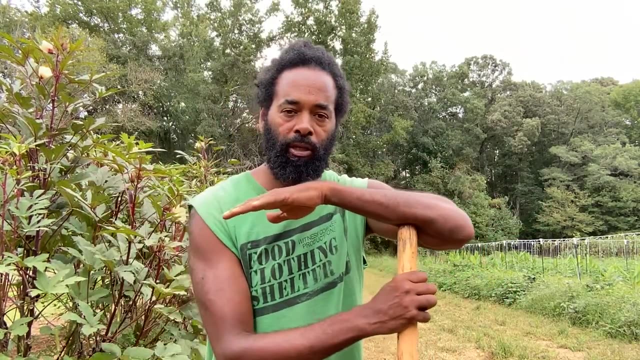 When we hear about the future use of past farm sites and realize that anywhere in our community that food production is being decreased And we don't see an equivalent increase In food production in a rural area close by or in the same area, Then it's saddening.